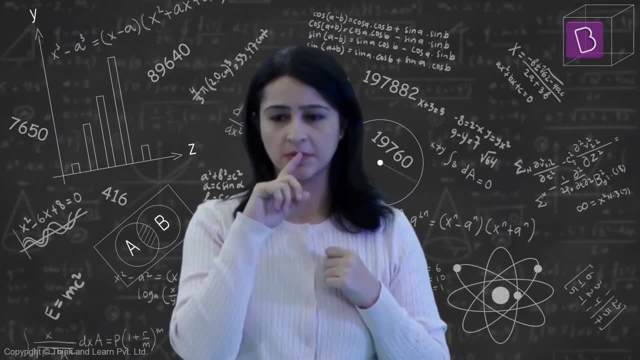 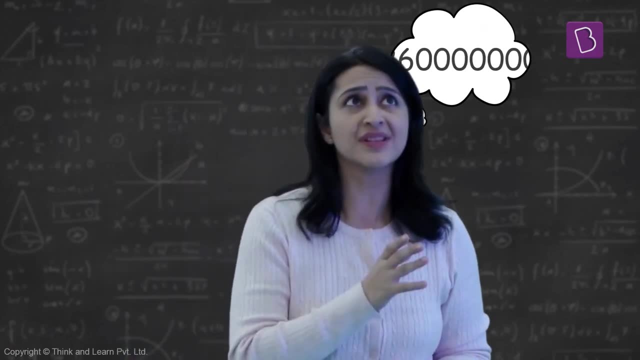 What's the hydrosphere? Okay, done So that's 12600000000…. I can't do it This number here. That's 162000000000… That's 1621000000000… 1621000000000…. That's 162100000000… 2625000… 2626000000000… 26250000000000…, 2625000000… 2625000000…, 2625000000… 2625000000…. 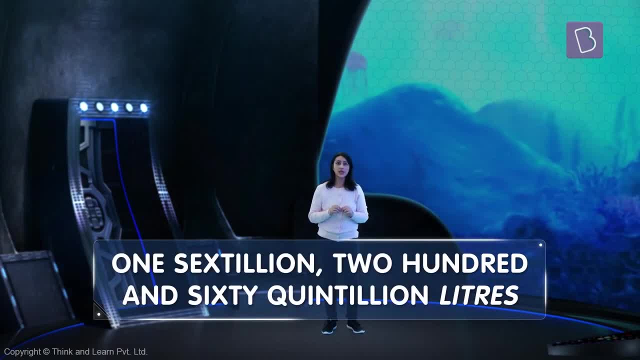 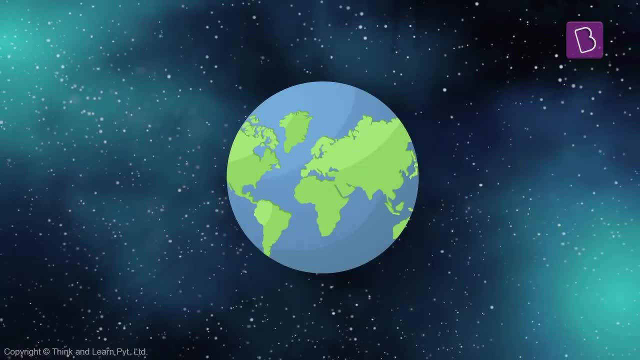 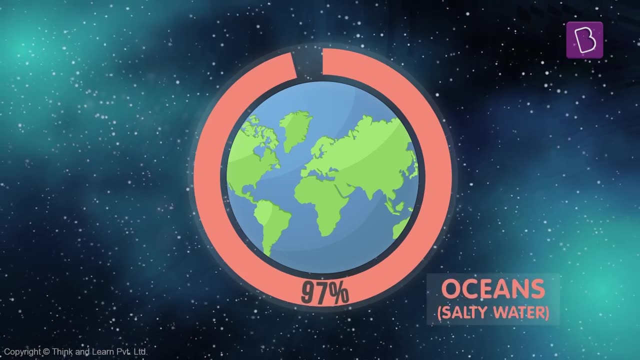 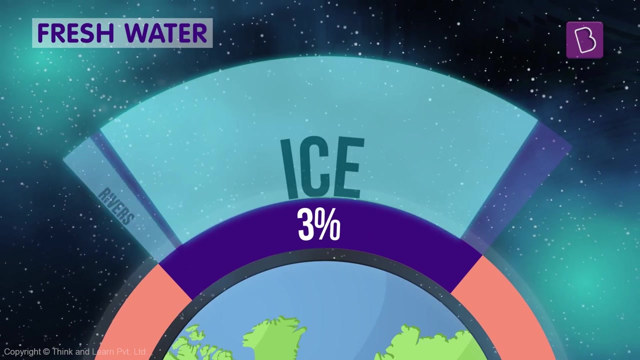 That sounds like a lot, But how much is it exactly? But guess what? Out of all this water, almost 97% of it is from the oceans- Salty water. The remaining 3% is non-salty fresh water that we find in ice rivers or under the ground. Most of all as ice. Yes, but that leaves very little for us, doesn't it? But then how come we haven't run out of water to drink? There are so many of us on this planet and we all keep drinking water. And then there are the animals too. 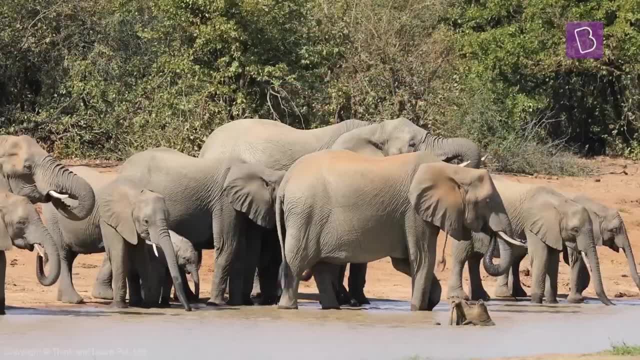 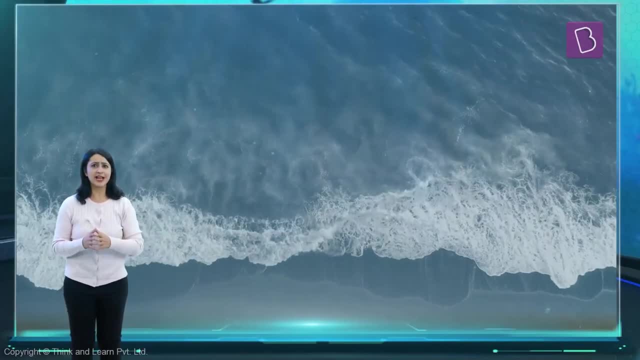 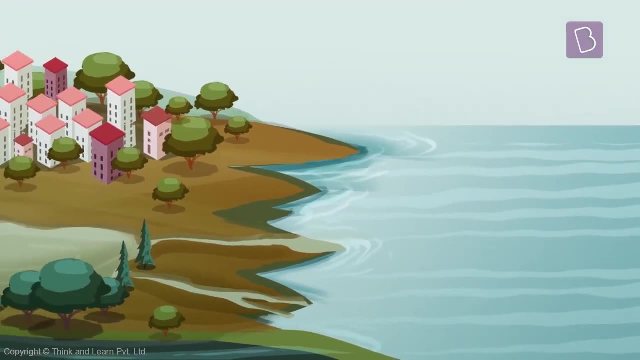 We should have run out of water a long time ago. Something doesn't add up. Well, it's time to tell you the story of water. Let's look at the water on the surface of the ocean. The sun's rays hit right into the water and the water heats up. 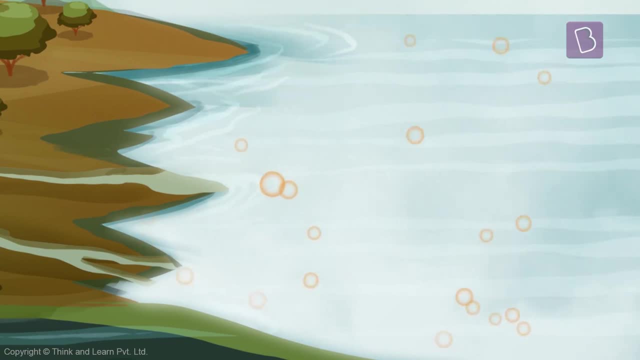 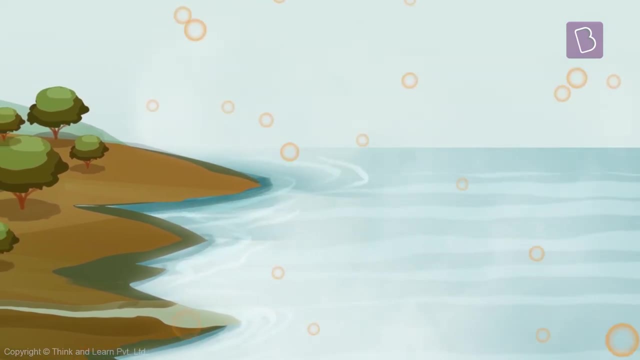 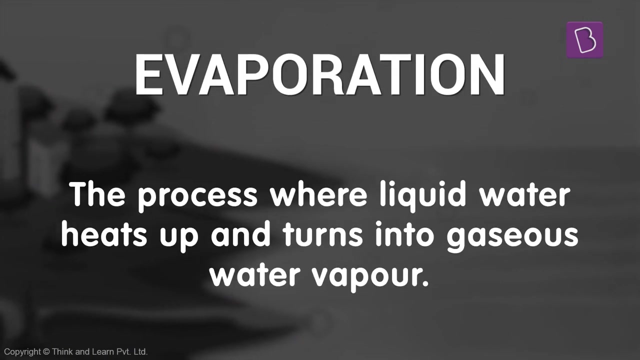 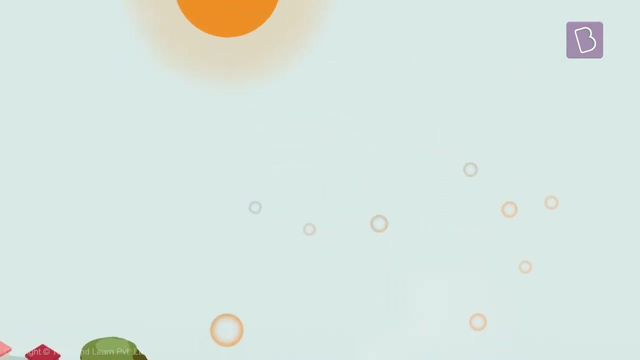 As it heats up, small particles of water detach themselves from the ocean and fly away into the air. This is called evaporation. This water travels all the way up to the sky and over time, cools down and starts forming little droplets of water. 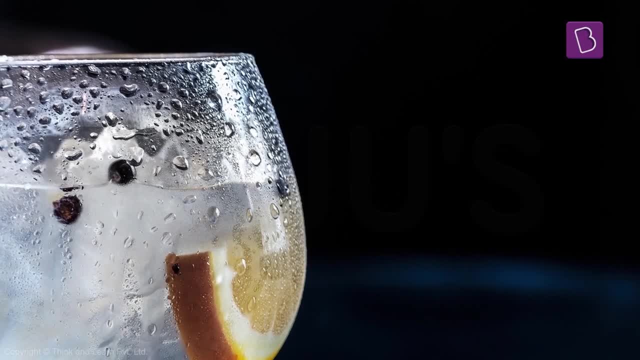 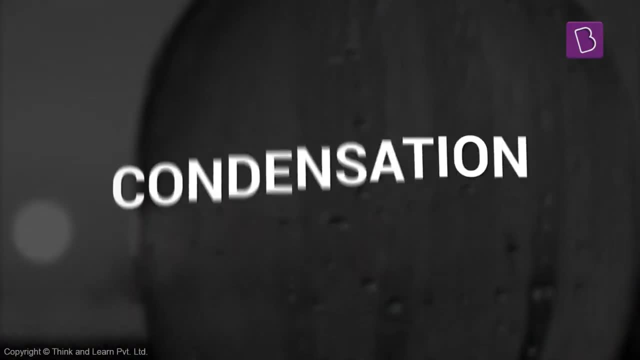 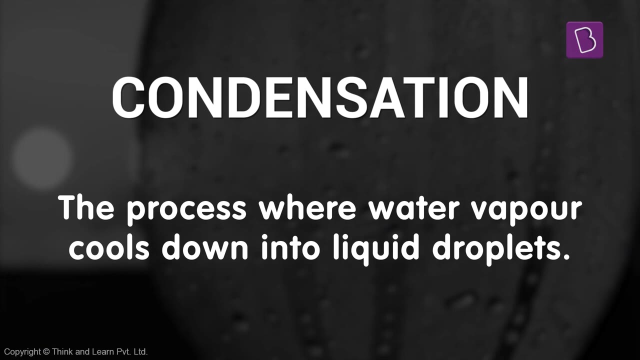 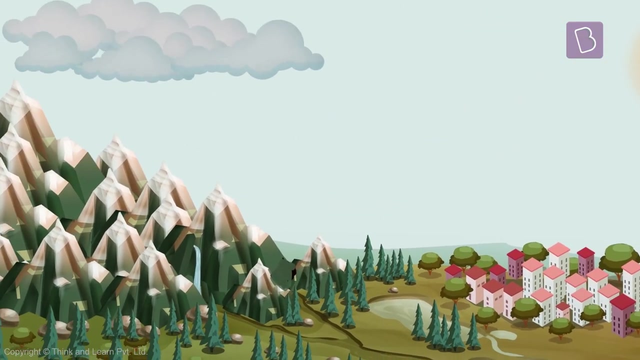 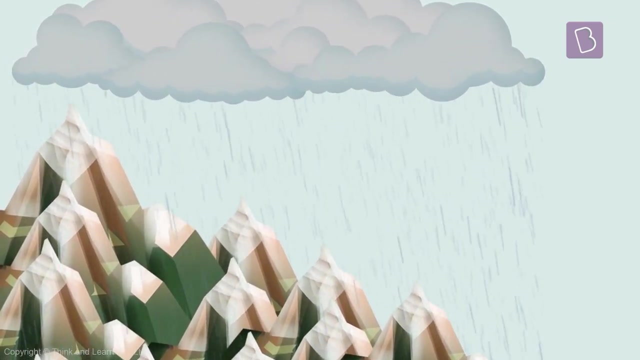 It's just like how water drops start forming on a cold water bottle if you leave it outside. Now this is called condensation. These clouds get heavier and heavier and eventually they give way to rain. All the water that went up now comes back down as rain or snow.